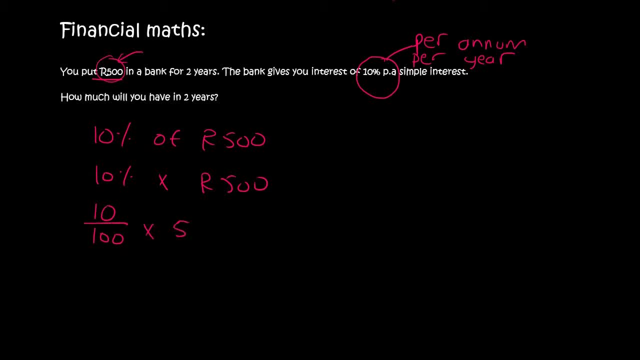 is 10 over 100 times 500 and that will give you 50 Rand, But that's 10% per year. So this is 10% per year. Your money is going to be in the account for two years And so 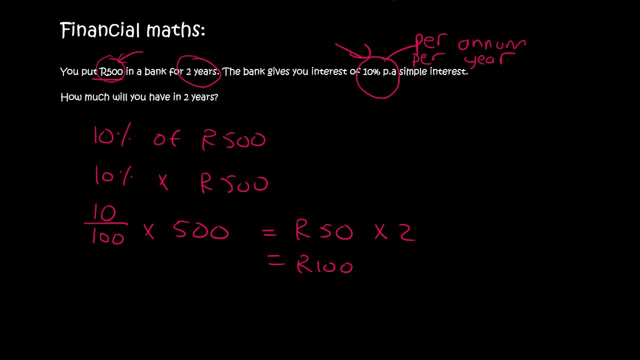 you will earn a total of 100 Rand. So when you go, look at your money in two years' time, you would have earned 100 Rand from the bank, And so your total would now be the 500 Rand plus the 100 Rand, And so now you have 600 Rand. Now, thankfully, we never have to go. 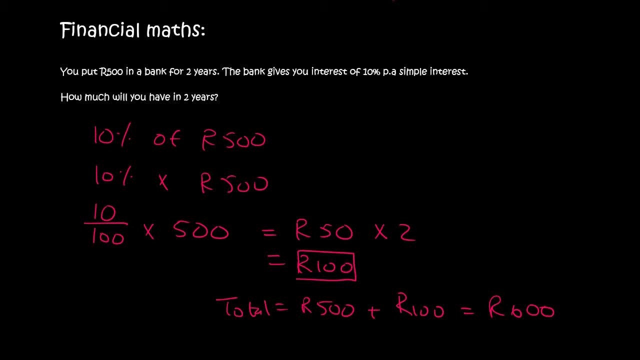 calculate it like this: This isn't the 15% of 500 Rand, This isn't the 15% of 500 Rand. century guys. we've got a formula, so this formula over here does all of that for us. so a is your final amount, P is the starting amount, I is the percentage and. 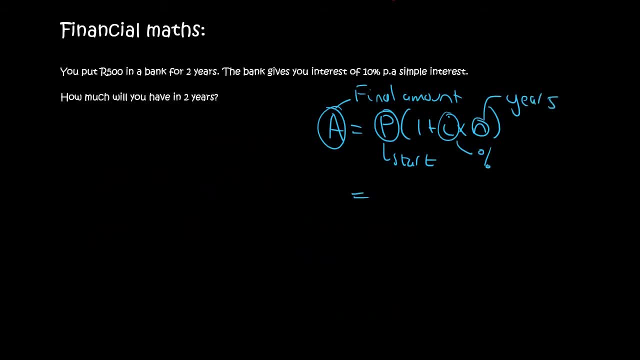 n is the. so check out. cool, this is P. well, that's your starting amount. you started with 500 rand. your percentage is 10%. now you can either type in 10%. some calculators have a percentage feature. the most popular calculator that students use in South Africa is the Casio. that one does have a percentage. 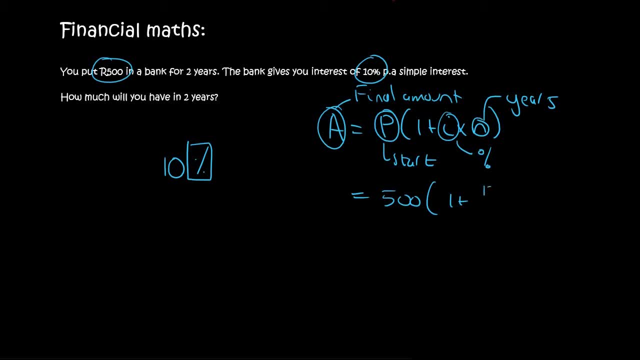 you must just look out for it, or what a lot of students like to do is they say 10 over 100, and then the number of years is 2, and so you literally just go type all of this in on the calculator and then you get the percentage of the. 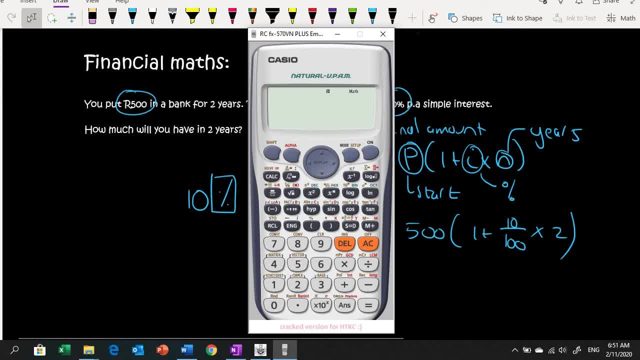 calculator like that, and so I'll quickly show you what it looks like. so we're gonna type in the 500 rand. you say bracket and you say one plus. oh no, if you want to use the percentage, you would say ten, then you would say shift and 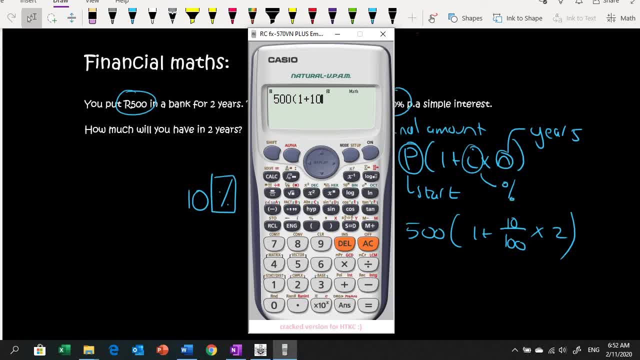 then over here, where's it now? there's a percentage sign just above the 8 and the 9. can you see there's a low percentage that you'd push that. but if you want to do the other method, you would say 10 over 100. 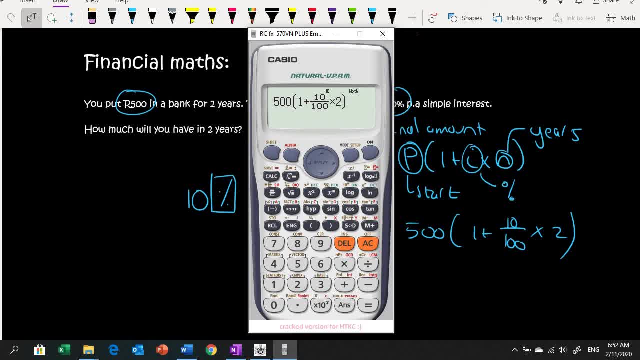 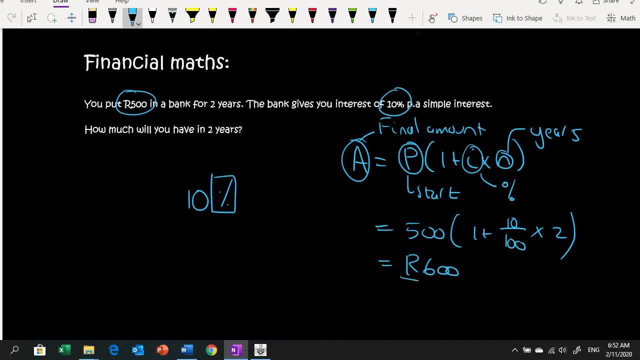 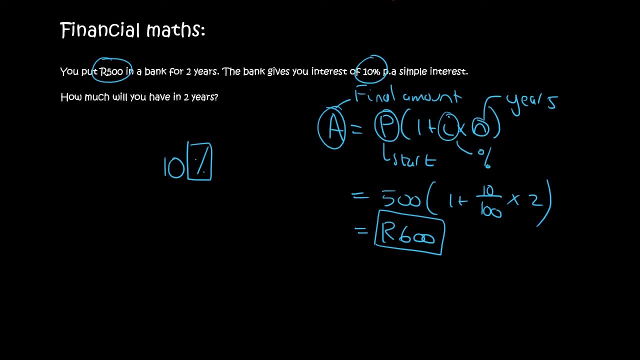 then you say times, and then there's two years boom: 600 Rand, and that is exactly how much we had earlier: 600 Rand. so this answer, or this formula, gives you the final answer and you don't have to go add the interest or anything like that. so just be careful, though. so you started. 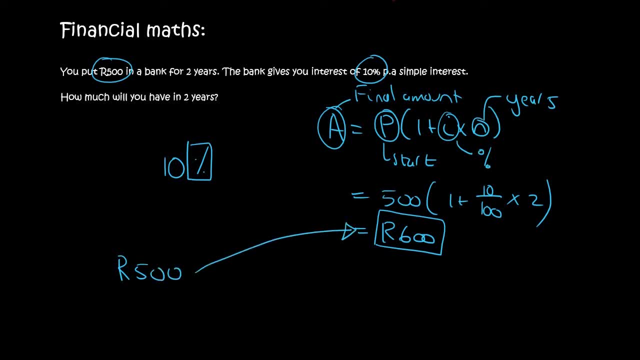 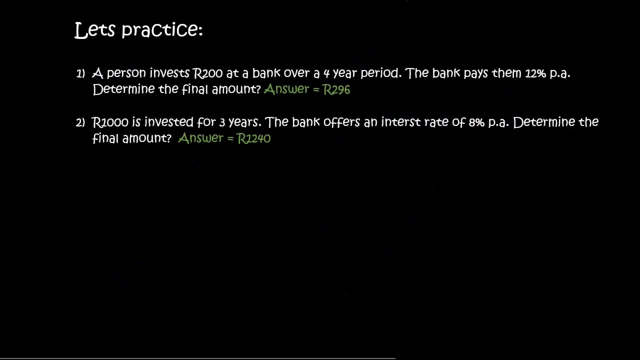 with 500 Rand it becomes 600 Rand. so how much did you actually earn? or your interest will be the 600 Rand minus 500 Rand, and so you earned 100 Rand. that's how much you actually earned at the bank. you didn't earn 600 Rand because you already had 500 Rand to start. all right, 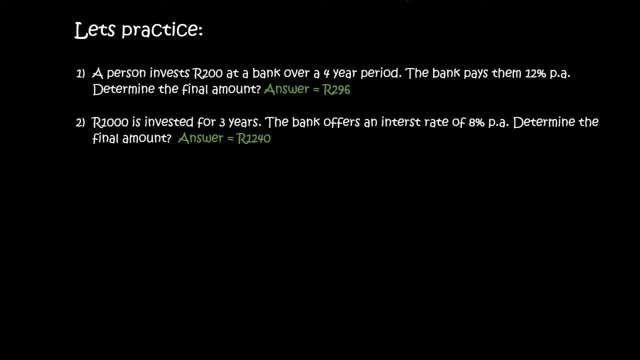 so here's two practice questions. I would highly advise you pause the video quickly and try them yourself. You have got the answers given to you, so go ahead. good luck. all right, so the way that this would work is for number one, it says a person invests 200 Rand at a bank over a four-year. 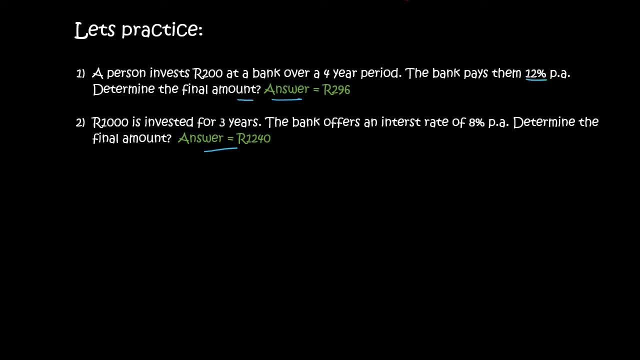 period the bank pays them. 12% determine the final amount. okay, well, we know that. there's now this handy formula that we use, where P is always your starting amount, I is always the percentage where you can either type in 12% or you have to say 12 over a hundred, then the number of years. 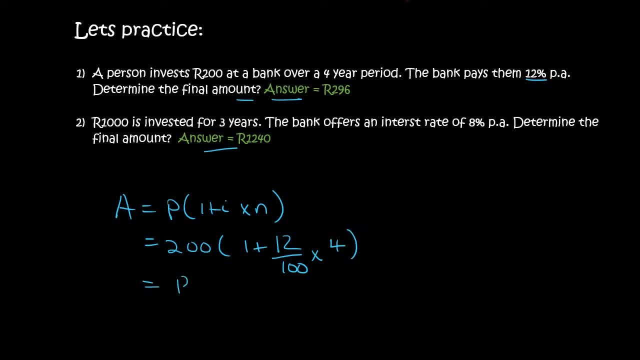 is four. you type all of that in on the calculator and you get 296, that is the total amount that the person has. how much interest did the bank actually give them? well, that would be 296 minus 200, and so the bank actually gave them 96 Rand. that's just for extra information. 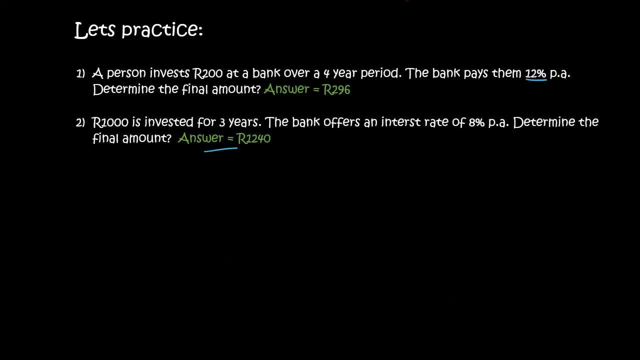 the actual answer is this one number two: 1,000 Rand is invested for three years, the bank offers an interest rate of 8% PA- remember, PA is per year- determine the final amount. so back to our formula where we, starting off with 1,000 Rand, the interest rate is 8%. so I'm just going to go.